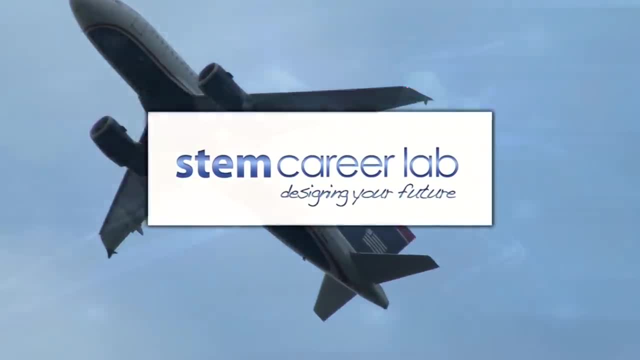 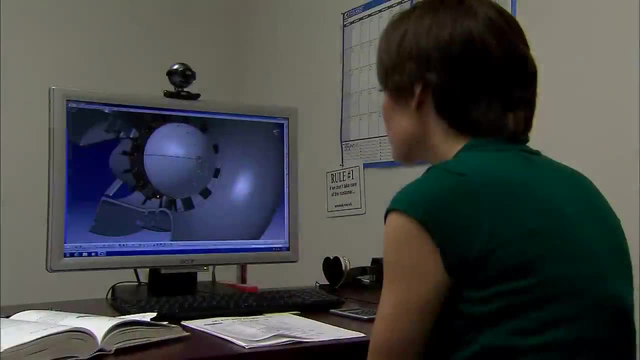 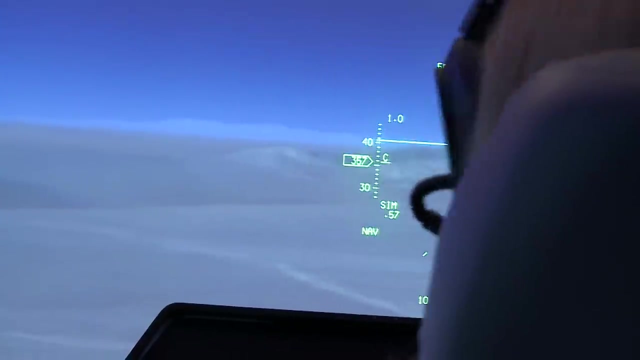 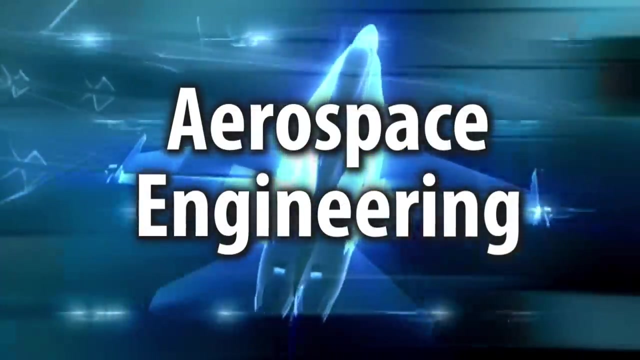 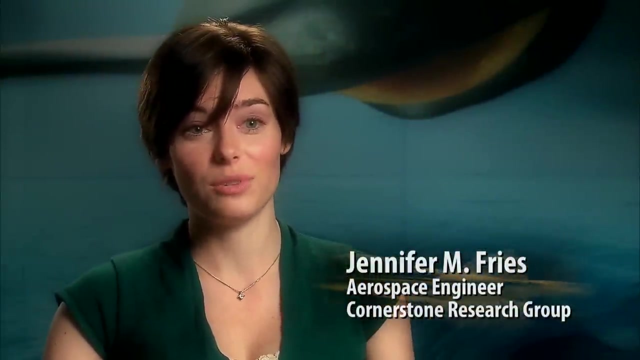 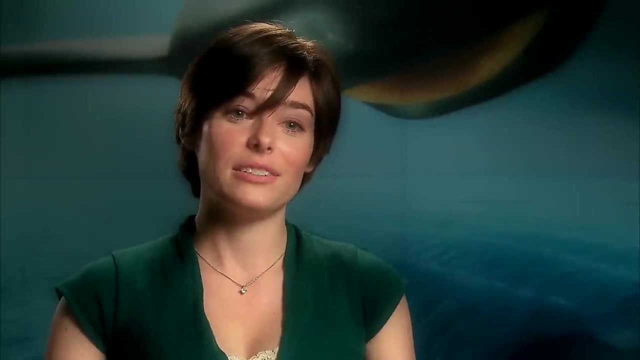 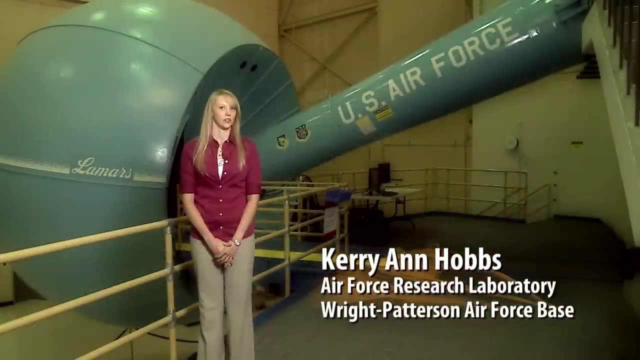 There's multiple types of aerospace engineers. There's aeronautical engineers, which are the engineers that focus on designing aircraft, things that fly in this atmosphere, And then there's aerospace or astronautical engineers that focus on spacecraft. Well, aerospace engineering is almost a very specialized form of mechanical engineering. 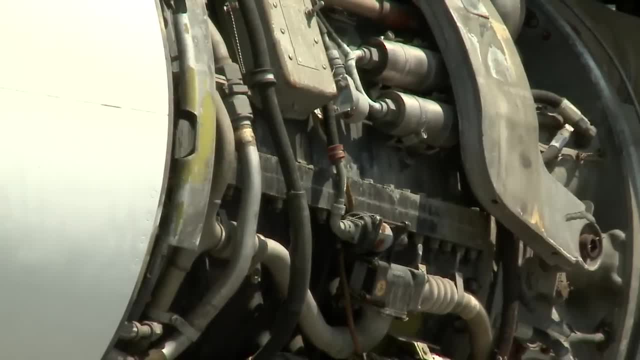 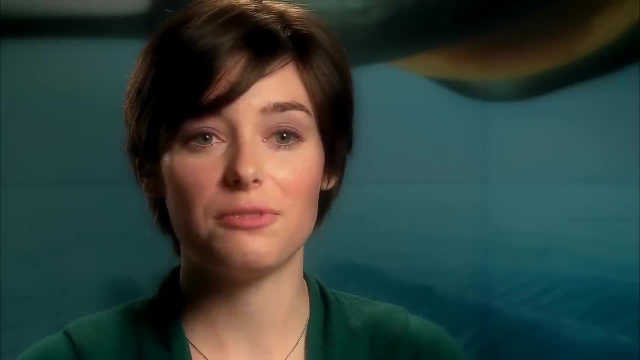 where you're looking at the structures of a system, the electronics of a system, the controls of a system. It's a whole system range of different things. There are aerospace engineers that focus solely on aerodynamics- how air flows over a surface. 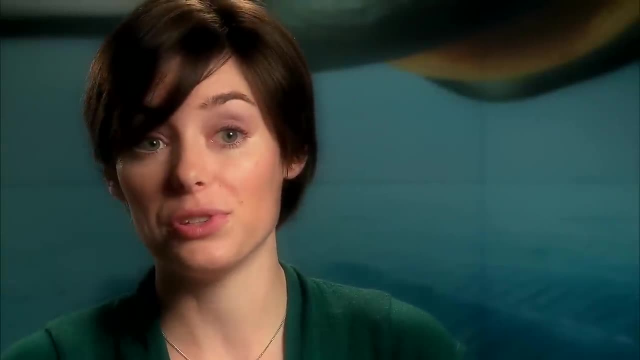 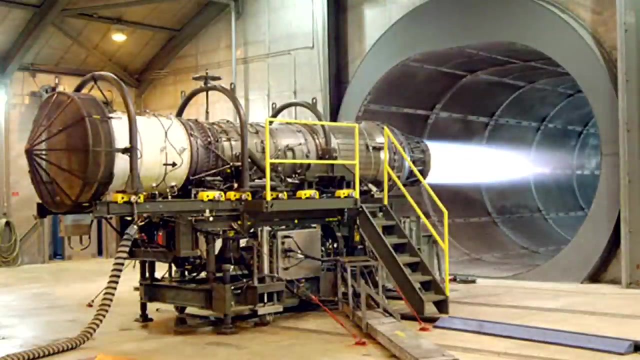 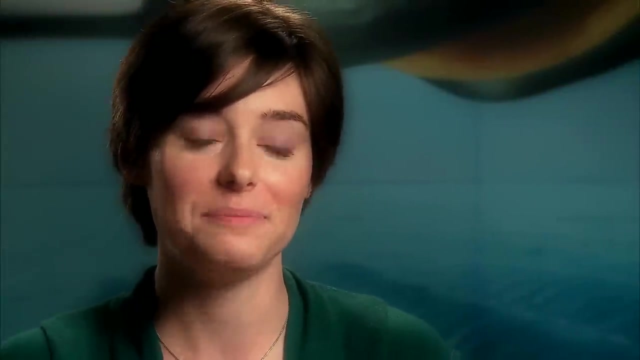 There's structural engineers that select what materials you're using. They determine what the inside of the aircraft looks like. There's also aerospace engineers that specifically focus on propulsion systems. They design the jet engines, They design rockets. They figure out how you get the aircraft from point A to point B. 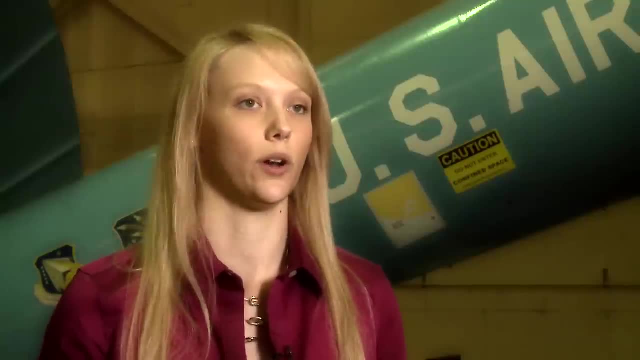 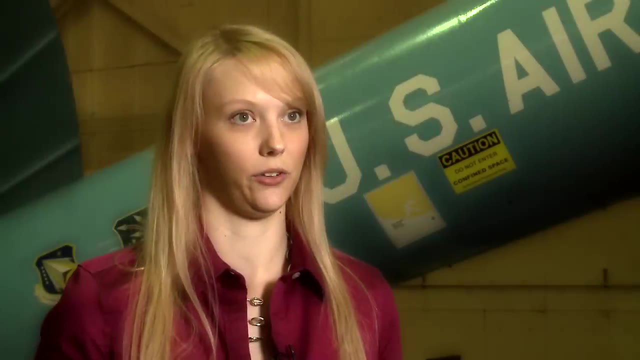 You really need somebody who maybe has a specialization in controls, working on a team, as well as somebody who is working in structures or somebody who's working in aerodynamics. They're all working together with their specialties, but they need to make sure that they're keeping. 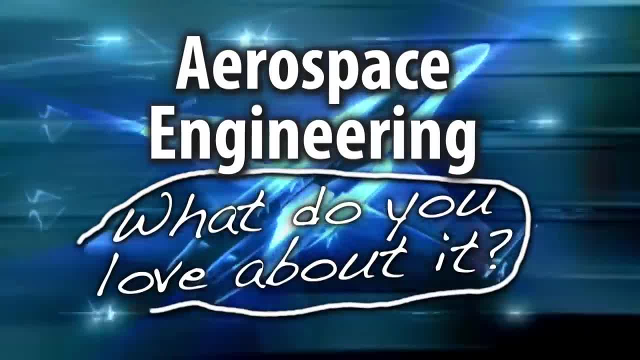 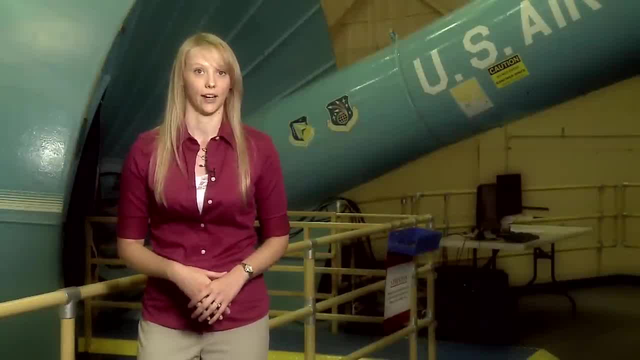 in mind the other specialties. When I was six years old, my parents took me to Space Center Houston, which was right near where I grew up in Texas, And when I saw all the work that they had done there, I was very inspired and I decided. 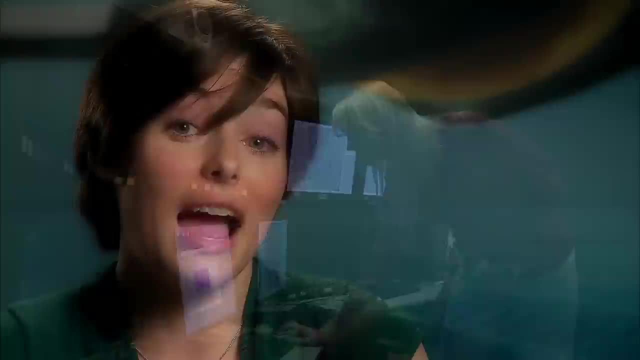 okay, this is what I'm going to do. I'm going to be an aerospace engineer one day. The thing I like most about my job is that every day, I can work on something different, And my degrees and my background, they're all different. 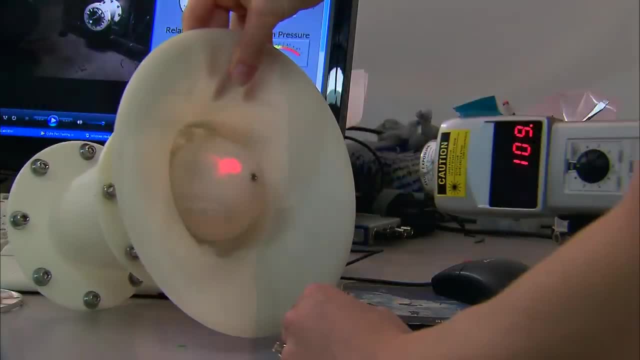 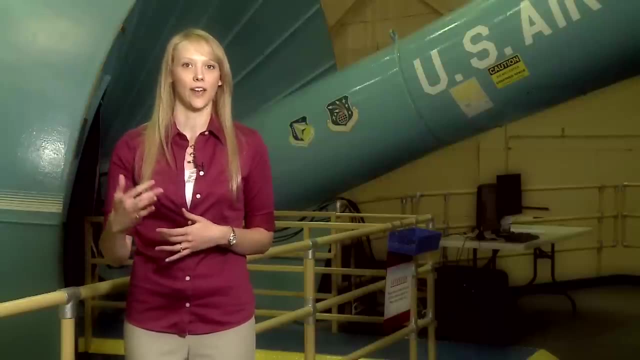 They're all different. My background allows me to create my own career and to work on things that I really am interested in. It's the next step of mankind. You're kind of on the edge of the envelope and improving people's lives and proving the 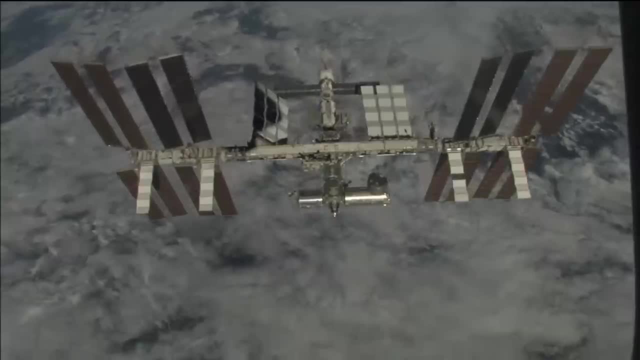 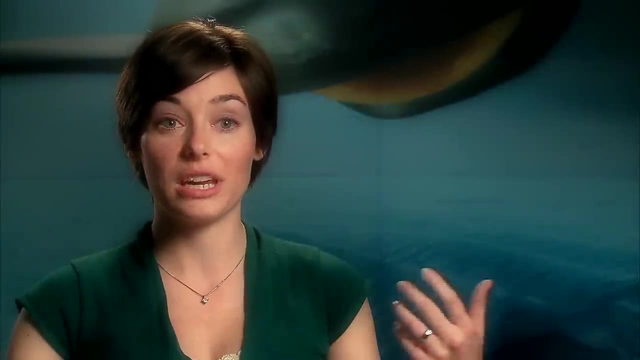 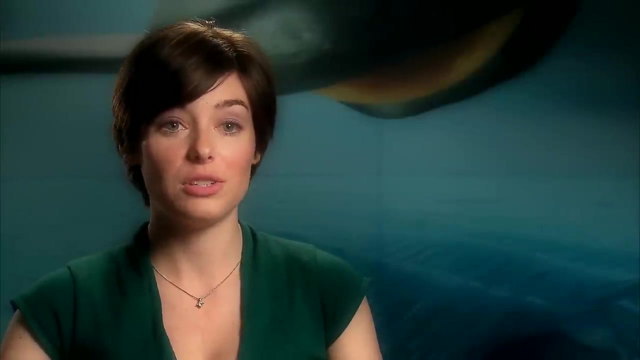 way that we can do things and taking technology that next step further. A lot of aerospace engineers work in the automotive industry. Aerospace engineers would design the shape of the car to allow for the airflow over the car to get you good efficiency. So here in our lab we're 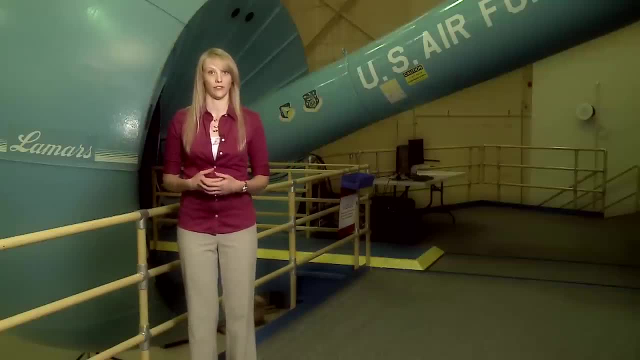 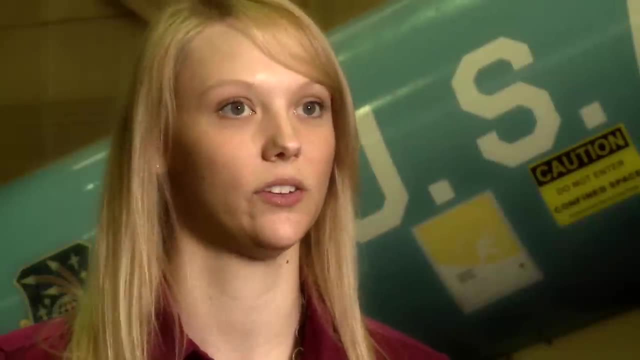 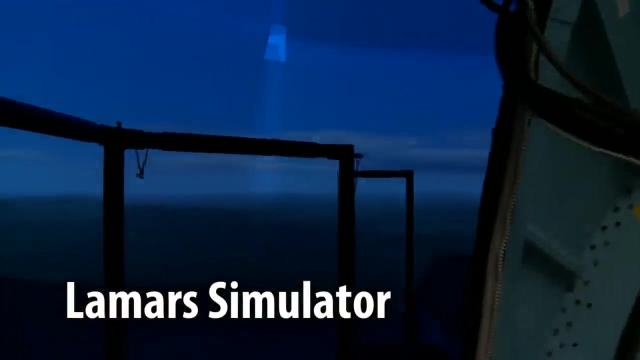 working on conceptual simulators, so we're looking at aircraft that don't necessarily exist yet and may not exist for another 20 to 30 years. We transfer all of the control laws and how it works, all of the aerodynamics, into a model on a computer that we then use to drive the Lamars, So a pilot can sit in there and 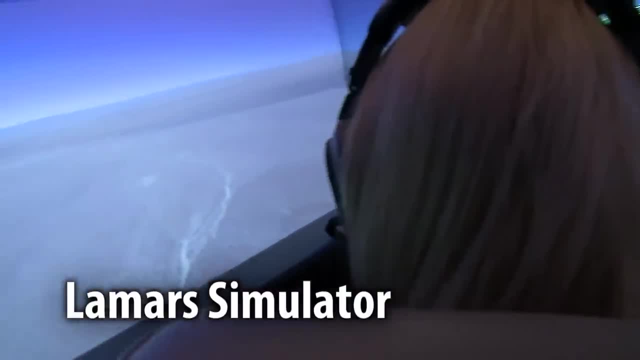 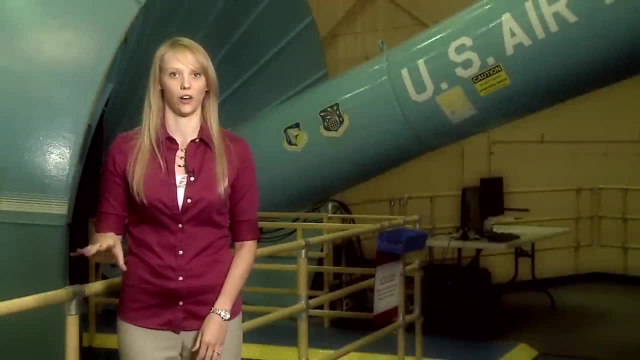 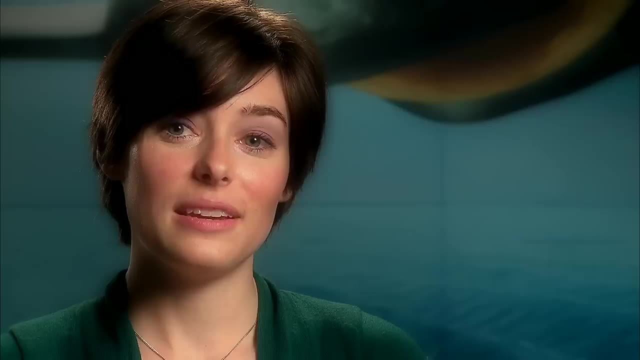 he can move the stick, and those reactions are then recorded and used to control the, the simulator or the aircraft in the real world. I'm also working on the automatic collision avoidance technologies program, which incorporates the automatic ground collision avoidance system. In my career I've done everything from designing parts on cars to designing aircraft. 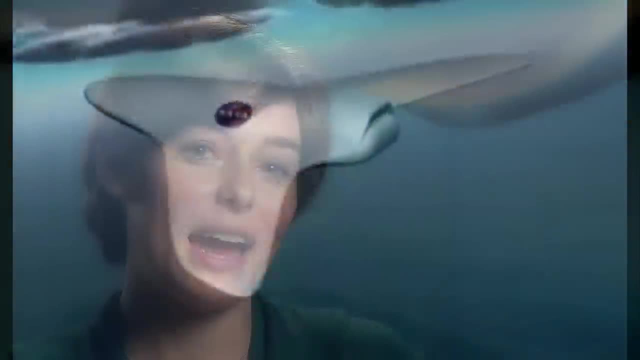 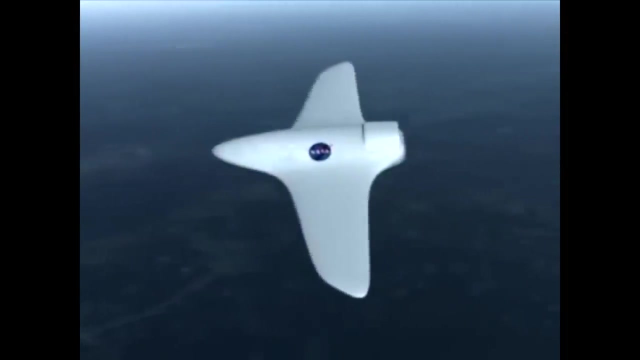 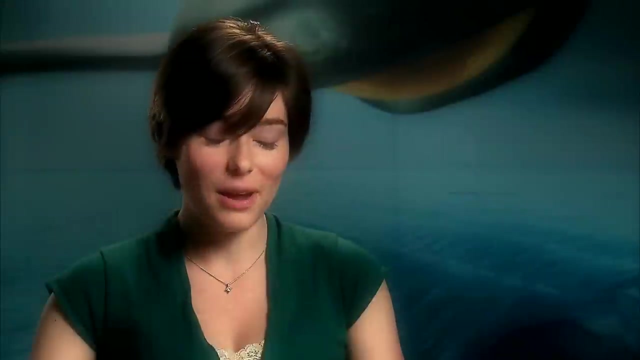 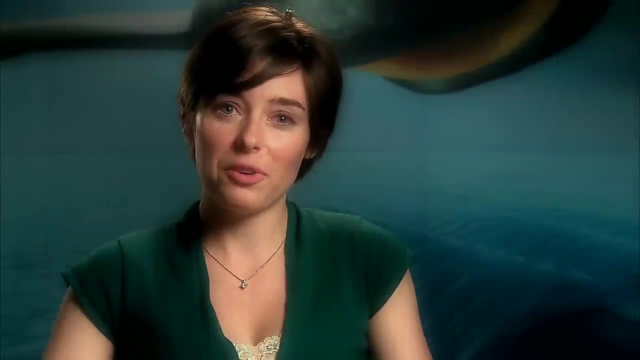 engines to designing morphing aircraft. Morphing aircraft design is aircrafts that can change shape during flight, which is the tricky part- to get an additional performance benefit. I guess I would be considered a rocket scientist, but I really don't like that terminology for myself. You do have to have a foundation math and science to be. 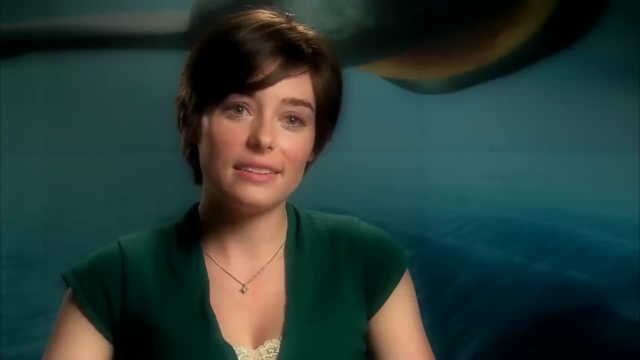 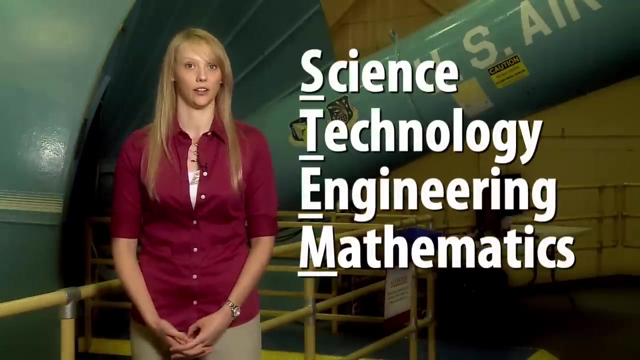 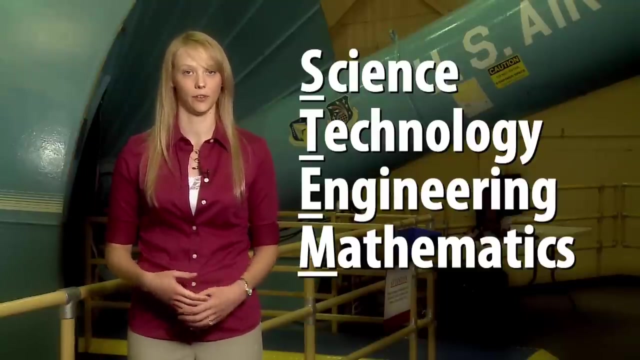 an engineer, but I think that it's a mistake to think that you have to be a genius. Aerospace engineering definitely fits within the science, technology, engineering and math fields. It is very heavy in the math. I'm using math and science concepts, physics concepts, potentially every day, Because 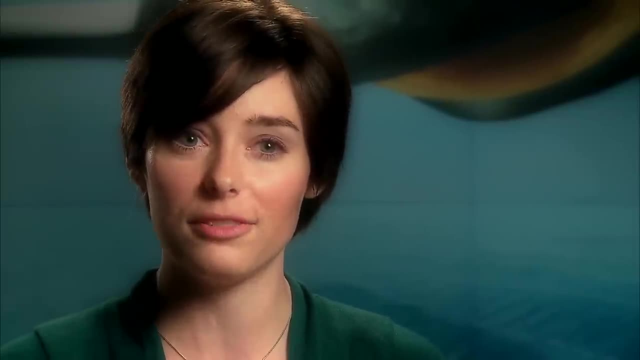 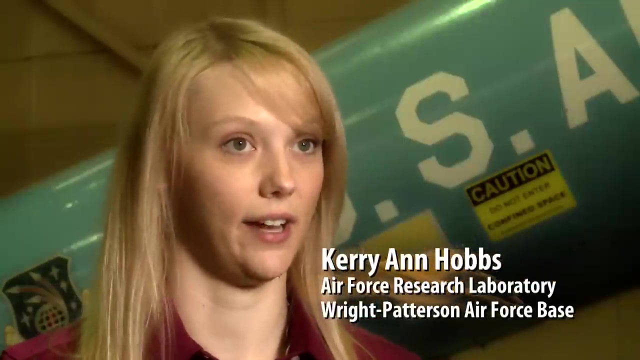 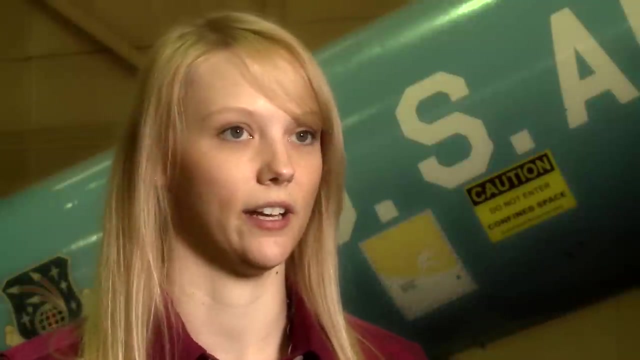 engineering is so based in a strong foundation of math and science courses. it's really important in high school that you start that foundation early. If you have the opportunity to take AP classes, be sure you're taking them, even if you're maybe challenging yourself and you're not making that A in that class that you 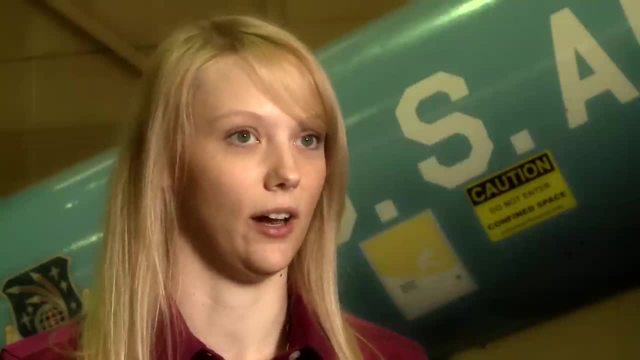 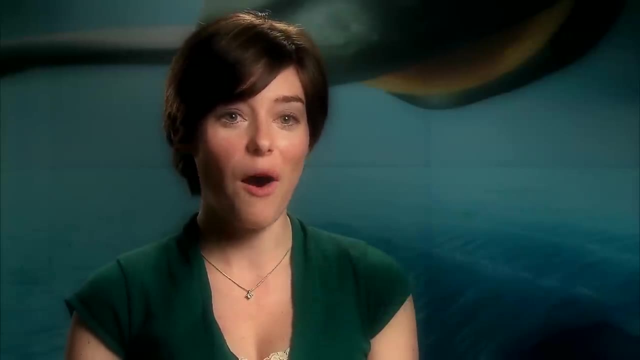 could make in a lower level class. take it because it will give you that really good baseline experience. I actually had people tell me, oh, you'll never use calculus, you'll never physics in your career. but honestly, all of my physics, calculus, chemistry books. 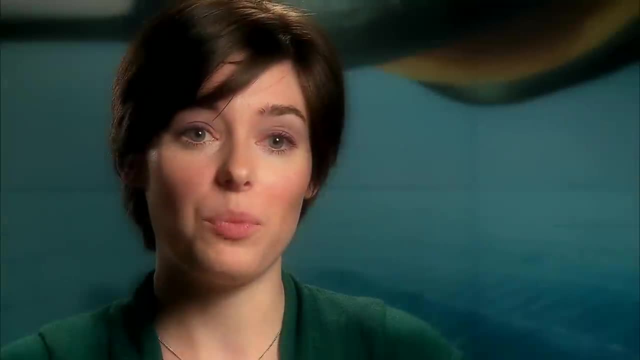 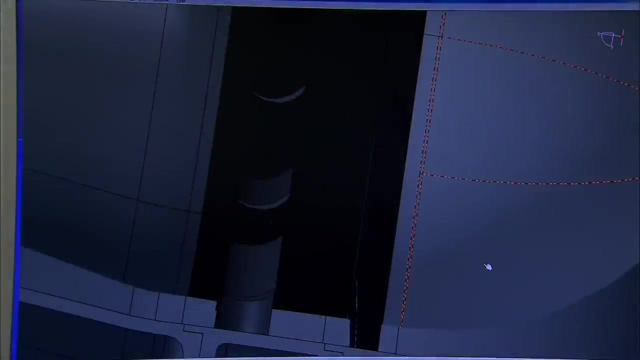 are on my bookshelf in my office. Geometry is a really good example. when you're trying to size a structure, you're trying to determine how big it should be, and you need to know the area of a trapezoid. Really, what's, almost more?